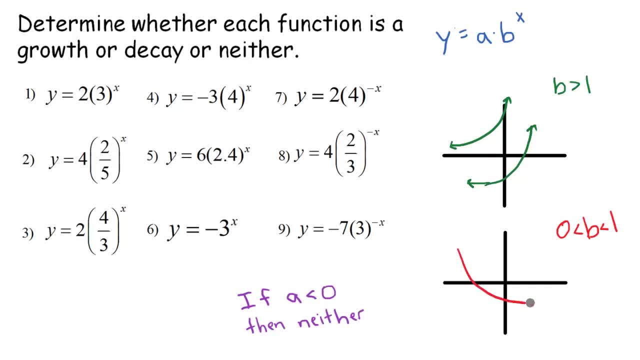 we have decays And that graph will look like this: As our X values increase, our Y values will decrease. It could be shifted, this could be another one, but they generally reflect this shape. If our a value is, which is the number in front of the b to the x power. if our a value 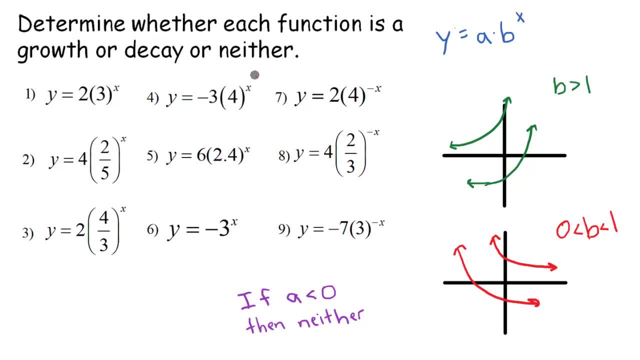 is negative, below zero, then it's not going to be a growth or decay, and that will look like this, or it could actually look like that. generally, these are just rough sketches, of course. Now let's go through one, through nine. 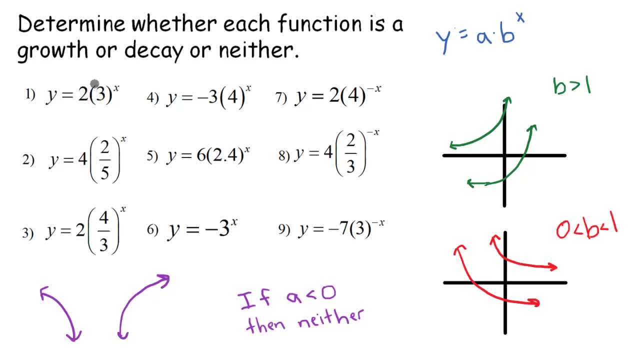 Number one: our b term is three, which is greater than one, so that reflects a growth. Number two: our b term is two fifths, which is between zero and one, so that's going to be a decay. Number three is four thirds: it's greater than one, so that's a growth. 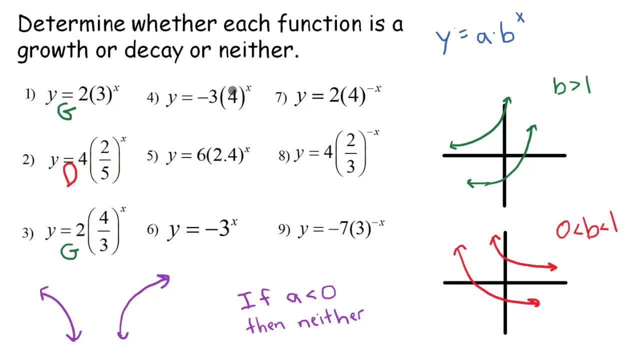 Number four. our b term is four, so that would be a growth because it's greater than one. but a- the value of a up in front here is negative three, Which is less than zero. so this is actually going to be neither. 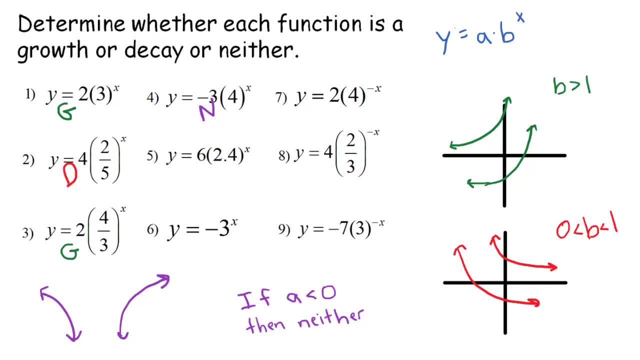 Number five. our b term is two point four, which is greater than one, so that's going to be a growth. This one right here will. you might think: well, what's our a term? We have a b that looks like negative three, but actually that b is positive three. 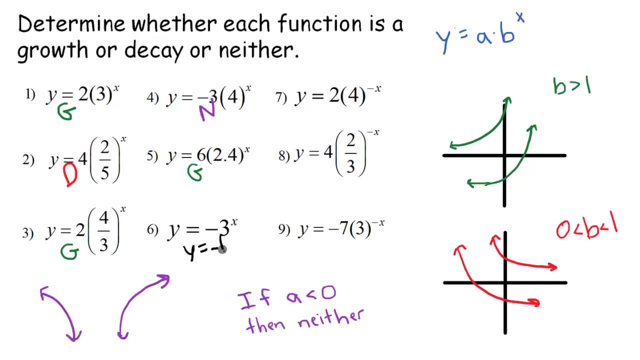 Our equation could look like this: Y equals negative one times three Negative three to the x power. So actually our a value is negative one, and we refer to this. If a is less than zero, it's going to be neither. 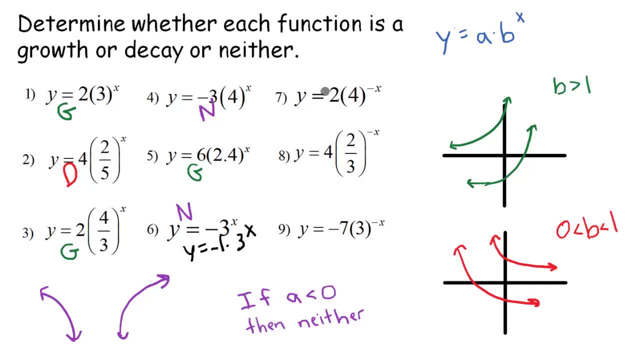 So let's label this as neither. Now, number seven, eight and nine all have a negative in front of the x's. Now, if we have a negative multiplier like that, we actually do the opposite of what it looks like. So in this case it looks like a growth, because our four is greater than one.